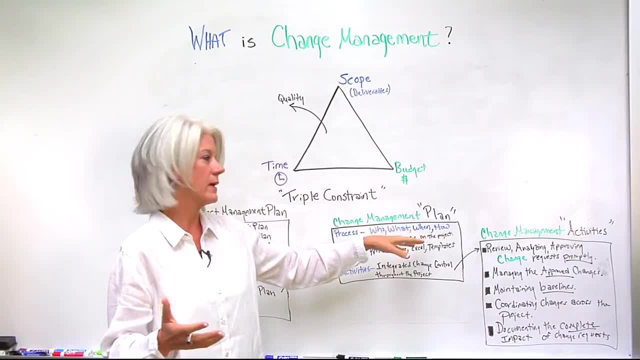 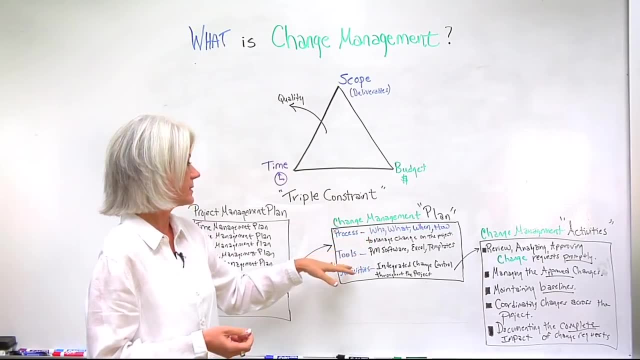 it's the process: who, what, when, where, how are we going to manage the changes on the project and throughout the entire project? It also includes the tools. What tools are we going to use? Are we going to use project management systems? 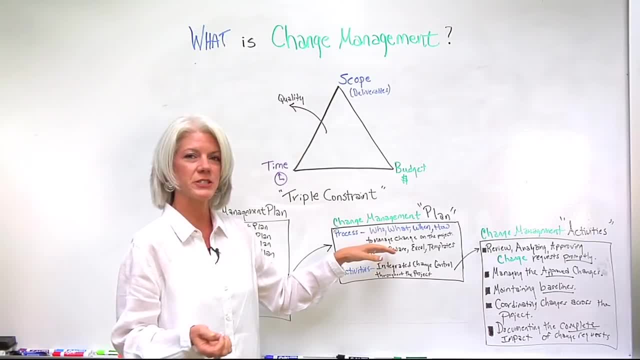 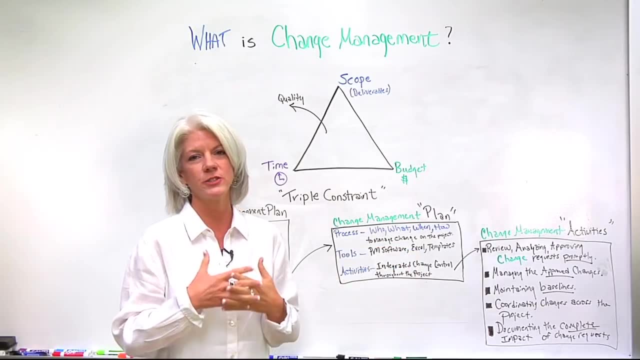 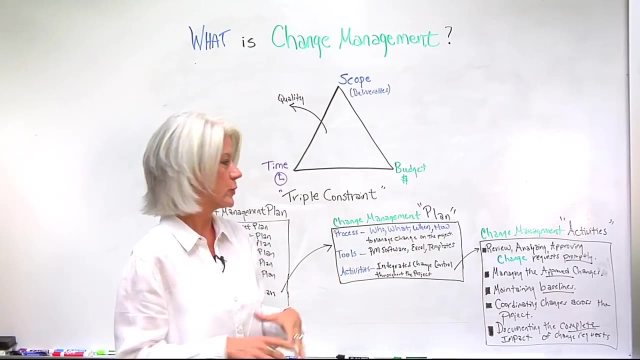 Are we going to use project management software? There are several great packages out there now of project management software that can automate a lot of this. Some groups or organizations choose to use Excel because that's what people have access to and to be able to track it among multiple groups. they have Excel. 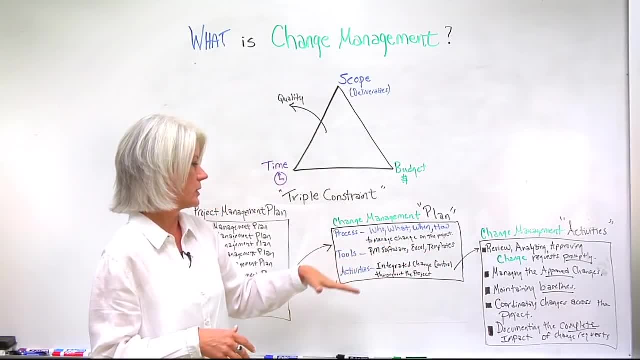 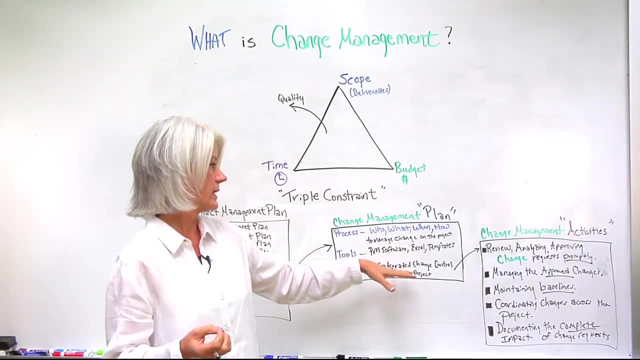 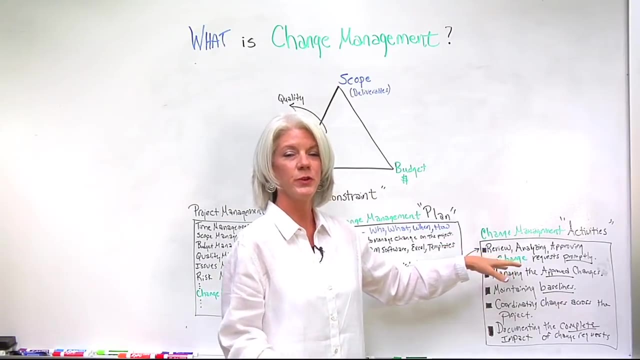 And then they use templates. So what are the tools we're going to use? And then the activities include things that how we the activities included for integrated change control throughout the project. So what are some of these activities? So the activities include reviewing, analyzing, approving change requests that come in, and doing that promptly. 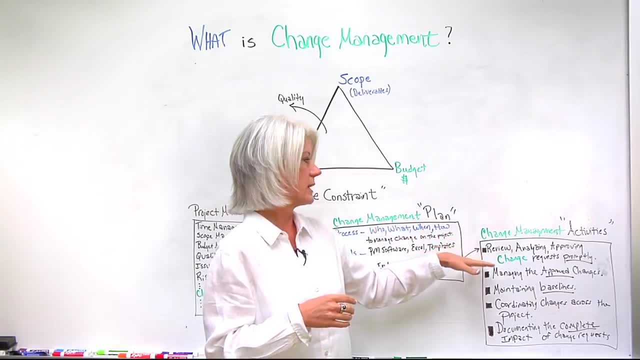 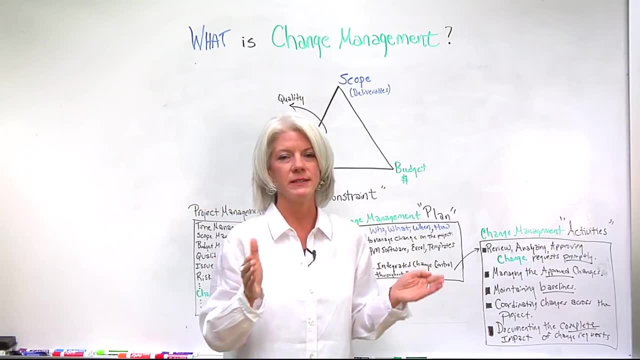 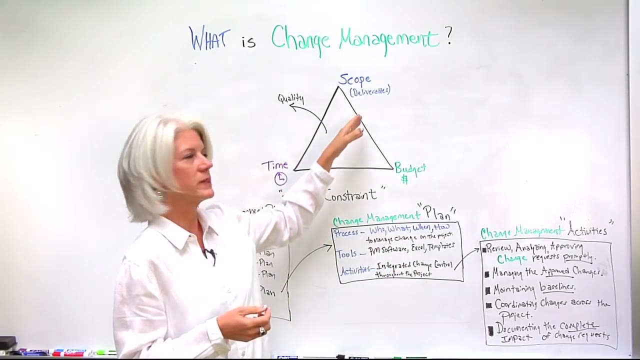 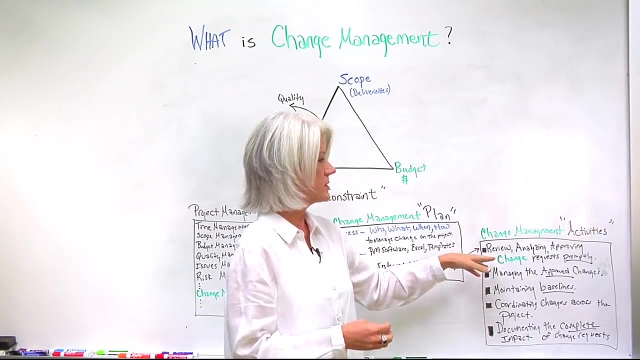 Because if things are left or if items are left, requests that come in, they come in for a reason, because it's things that may not have even been defined in the project or through execution. Maybe things are uncovered, Maybe things are occurring, Maybe things are occurring with the scope, the budget, the time, the quality that require changes to be submitted. 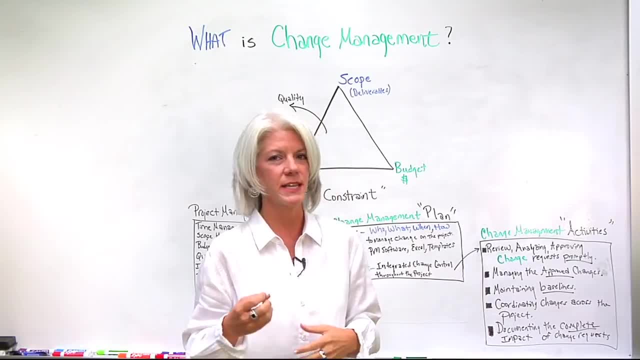 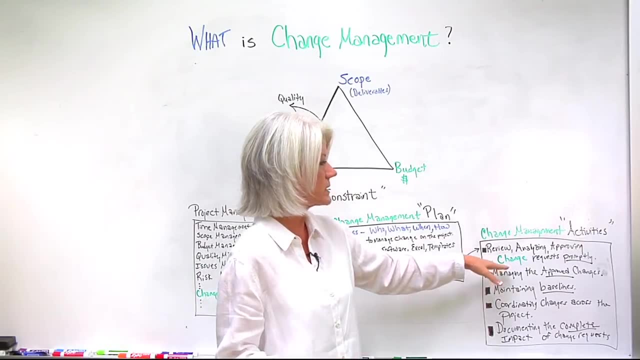 So those have to be handled promptly, Otherwise, if things are left unattended, it could have a negative impact on the project. It also includes activities such as managing the approved changes, So once they're reviewed, analyzed and approved, they need to be managed appropriately. 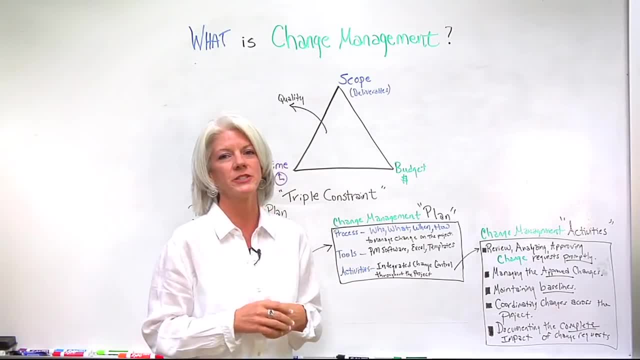 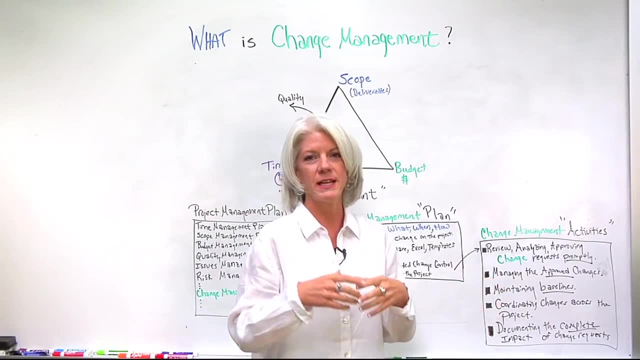 And then maintaining the baselines. I've said in several of the other whiteboard sessions, the difference between a failed project and a successful project sometimes has to do with something as simple as re-baselining the project, Because when changes are approved formally through your change control board, 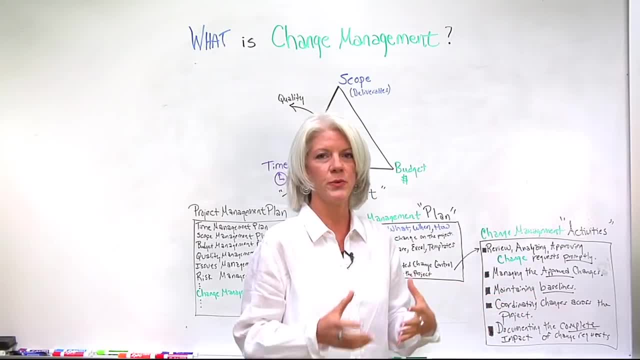 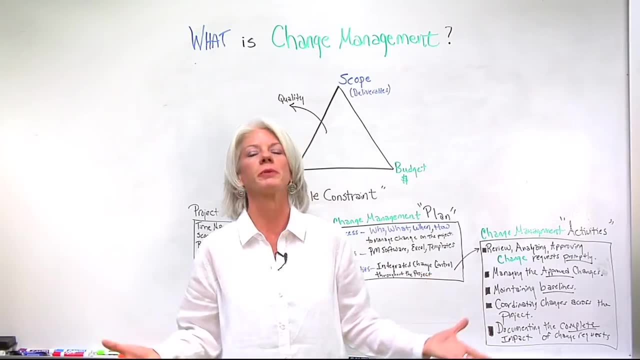 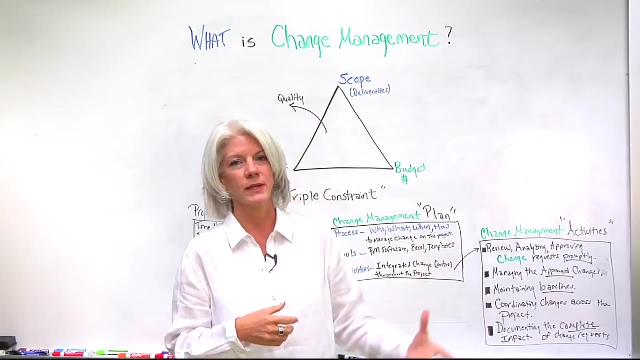 then that gives the authorization to go change the baseline, And then so it also includes coordinating changes across the project. So when changes are approved, a lot of times it may impact other groups, other organizations, whether they are inside, outside of the project or the organization.